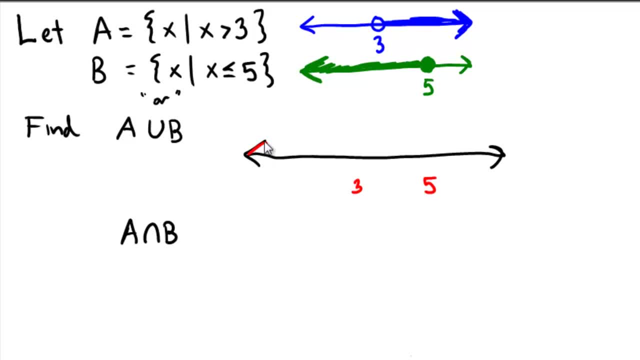 The whole set of numbers from negative infinity to infinity. The numbers that were located here were shaded by the bottom graph. The numbers that are in between 3 and 5 are shaded by both the green and the blue, And the numbers that are located above 5 are all shaded inside of the blue picture. 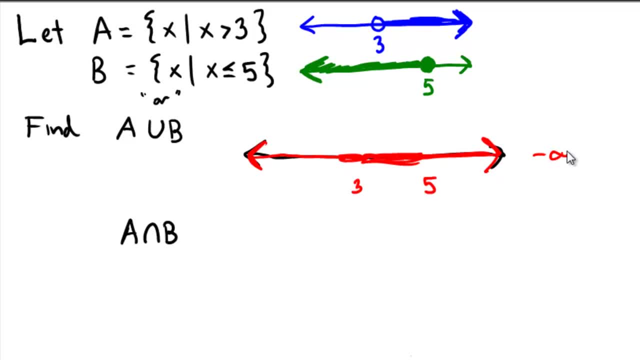 The top one, So the interval. the answer to this would be all numbers, from negative infinity to infinity. On the other hand, if we consider A intersect B, that means the word, and So now you're looking for ones that are shaded in the top and in the bottom. 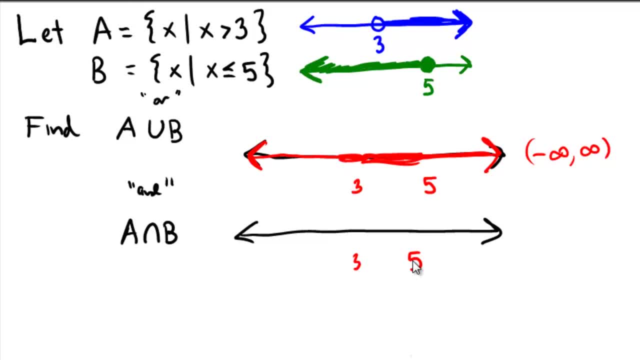 So, again, using 3 and 5 as placeholders, we can see that we don't shade things to the left of 3 because they're only in the green. We don't shade objects bigger than 5 because they're only shaded in the blue. 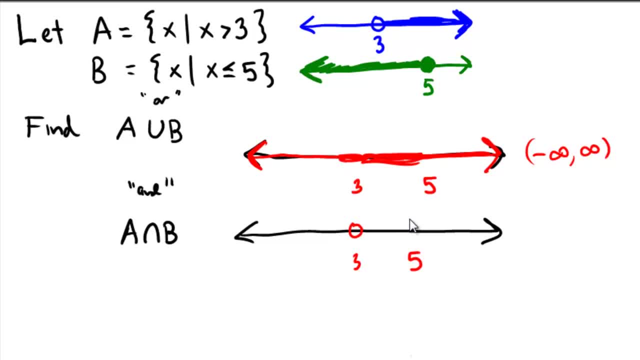 The numbers that we'll shade will be 3,, 5, and in between, Because by looking at both of my number lines, I can see those are both shaded top and bottom. Okay, a little bit more quickly, let's look at C and D here. 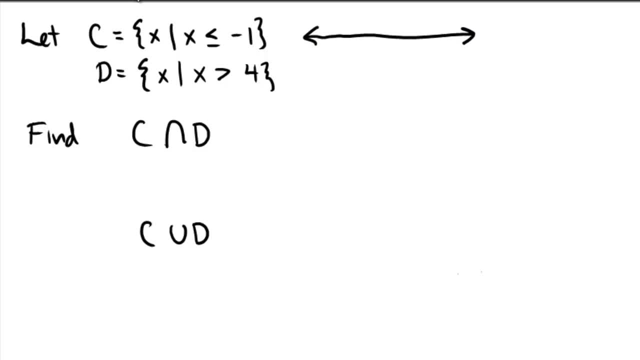 So C, the interval that is supposed to be less than or equal to negative 1.. So here's negative 1, solid dot and left. And then for the second example, or for set D, we want it to be bigger than 4.. 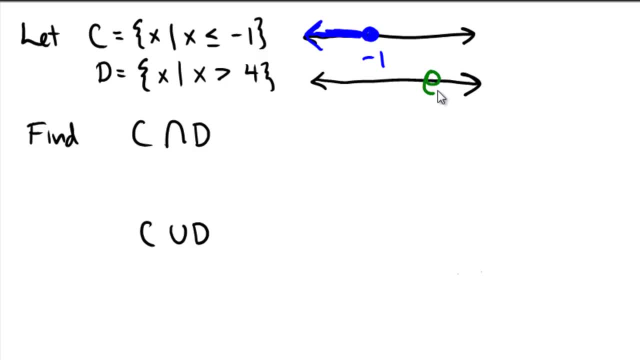 So again, a number, line 4, with an open dot and shading to the right. So now, what are the answers to the two questions? Well, the first one was intersection, which would be the things that are shaded in either the top or both the top and the bottom. 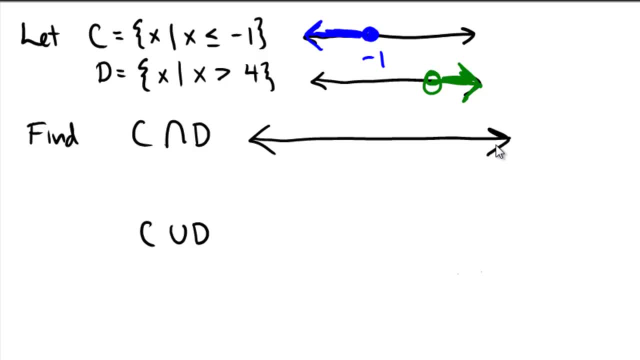 But notice that nothing is shaded in both the top and the bottom. So that means the answer here is nothing. No numbers are shaded, Absolutely nothing at all, And that's the empty set. In the bottom one we have C, union D. 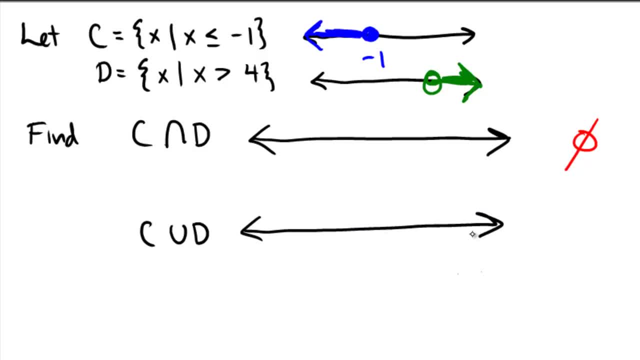 So here we want the ones that are shaded in either the top or the bottom. So top blue gives us the numbers from negative 1 on down, And the top in the green gives us the numbers going from 4 and upward. 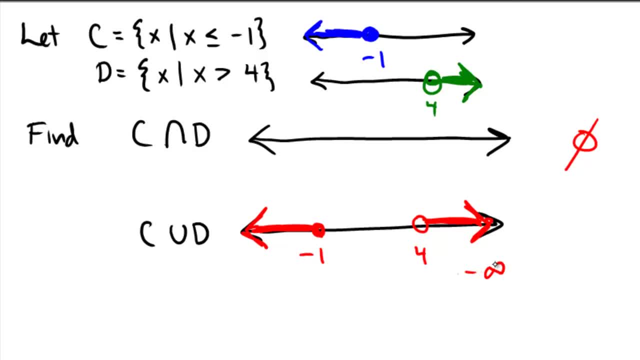 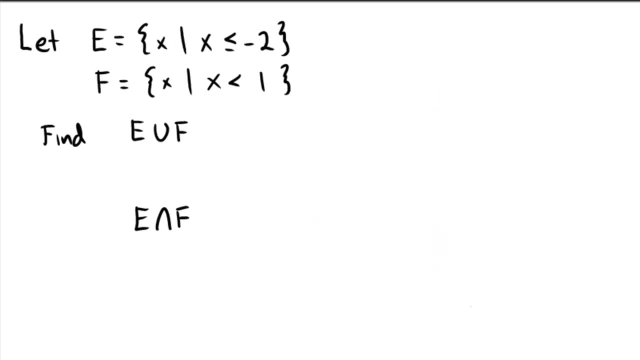 So the answer for the union would be negative 1.. So it would be negative infinity up until negative 1, and unioned with 4, off to positive infinity. So now, why don't you pause the video and try one on your own? Here's an example: E and F. 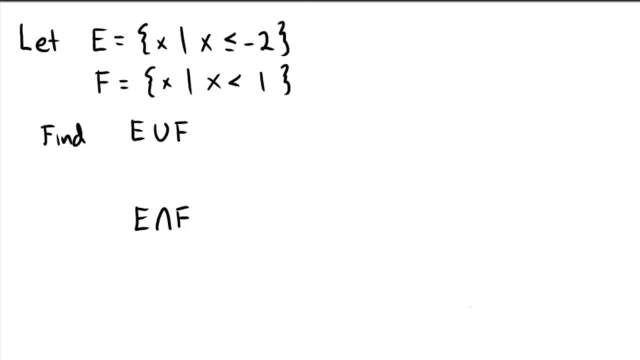 Both of these are going less than So, assuming you paused the video and tried it out on your own, let's try to do it together now and see if we get the same answer. So two number lines, Top one in blue, will go to the number negative 2.. 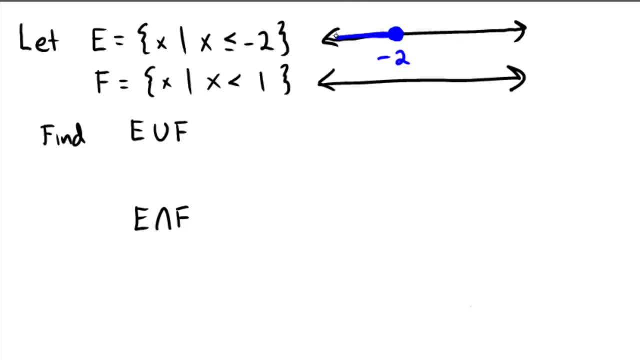 Less than or equal to. So we'll shade and shade to the left. The green one, the bottom one, would be x less than 1.. So we'll go to 1, put an open dot and shade to the left. 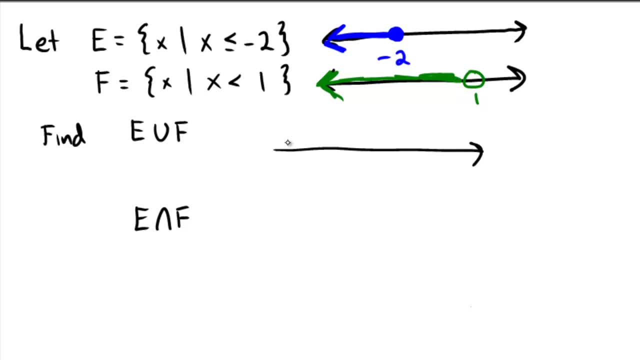 So when we bring these together into our union and our intersection, the union, which is the OR, means that we need things that are shaded top or bottom, So we will be going to 1. And below, Because notice that the numbers below negative 2 were shaded by both. 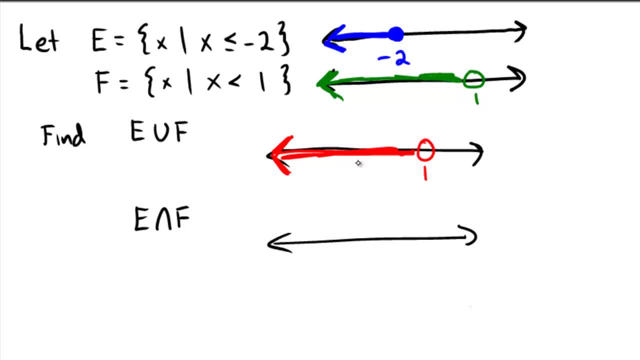 but the numbers that are less than 1 were shaded by the bottom only. but that's okay for the OR. On the other hand, for the AND, we wish to take all the things that are shaded in top and the bottom simultaneously. So for that one we'll go to the negative 2, put a closed dot and let that shade to the left. 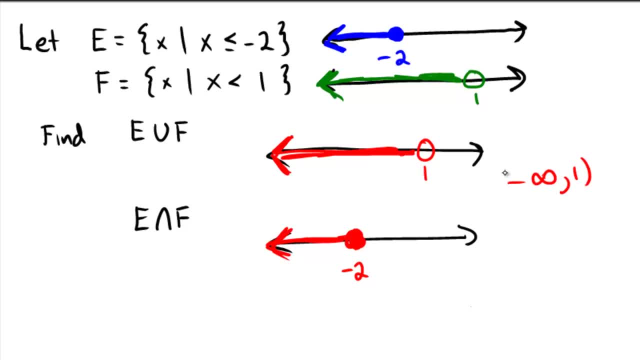 In interval notations. these would be negative infinity up to positive 1, open and negative infinity up to negative 2, being closed.